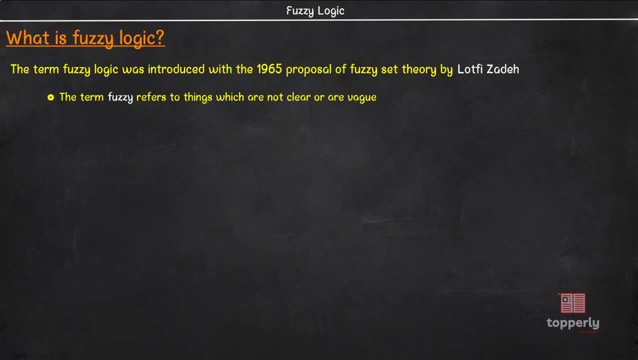 many times we encounter situations where we can't determine whether the state is true or false. In such cases, Fuzzy Logic provides a very valuable flexibility for reasoning, So it resembles human reasoning in many ways, and hence we can consider uncertainties or inaccuracies of any situation. 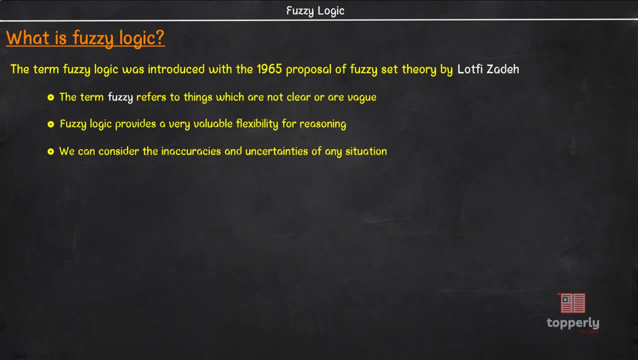 Now, before we dive deeper into this lecture, let us understand what is CRISP value. The term CRISP means precise and it deals with values. that has a strict boundary that is true or false. The value should be either true or false to be called as CRISP value. 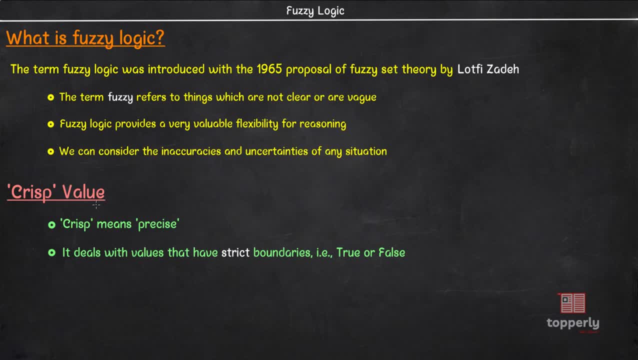 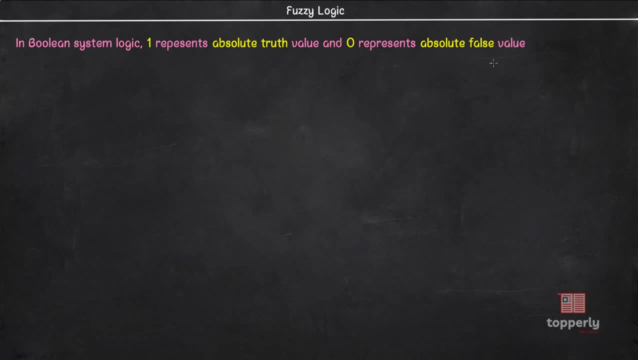 and it cannot contain any in-between values. Coming to Boolean system truth values, 1 represents absolute truth value and 0 represents absolute false value. That is, 1 is true and 0 is false. However, in the case of Fuzzy Logic systems, we have intermediate values present, which are partially true and partially false. So, in the case of Fuzzy Logic systems, we have intermediate values present which are partially true and partially false. So, in the case of Fuzzy Logic systems, we have intermediate values present which are partially true and partially false. 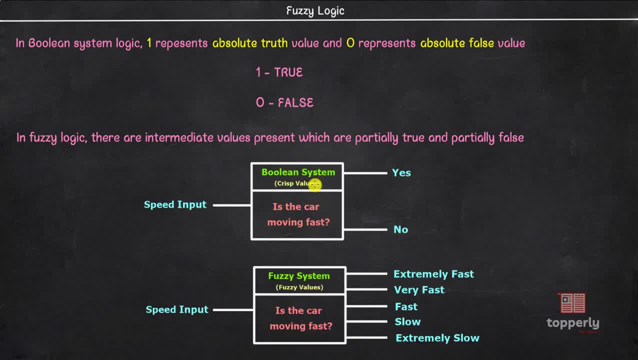 Now let us consider an example to show how Boolean system truth value works and how a Fuzzy Logic system works. In this question you can see that the condition is: is the car moving fast In the Boolean system having CRISP values? you can see two solutions: yes and no. 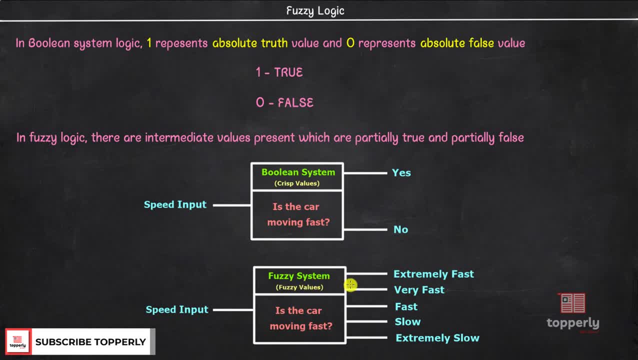 But in a Fuzzy Logic system with Fuzzy values, you can see that there are many solutions. The car can be moving extremely fast, The car can be moving extremely fast, very fast, fast, slow or extremely slow. So you can say that in a Boolean system having CRISP values, 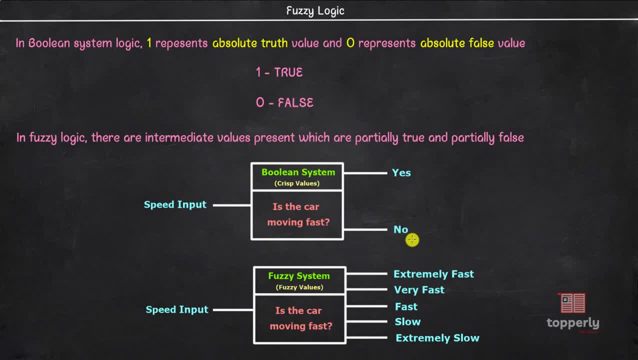 you only have absolute true value and absolute false value. But in a Fuzzy Logic system you have these partially true and partially false values. As you can see extremely fast, very fast and fast are somewhat close to the absolute true value. So you can say that these are partially true and partially false values. 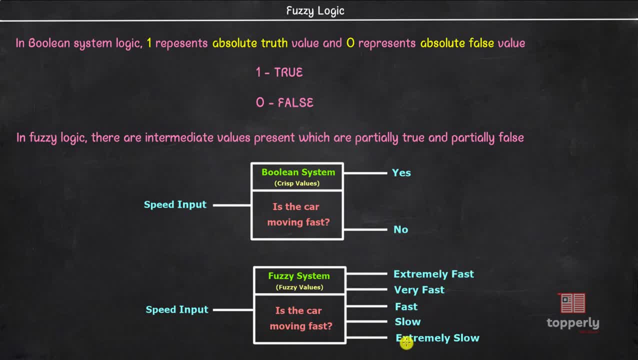 Similarly slow and extremely slow are somewhat close to the absolute false value. Therefore, you can say that these are partially false. So that is the basic difference between Fuzzy Logic systems and Boolean systems. Now we will talk about membership functions. 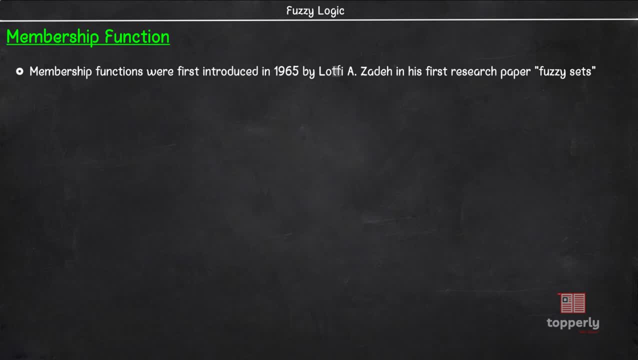 Membership functions were first introduced in 1965 by Lothvi Sade in his first research paper, Fuzzy Sets. They characterize fuzziness, that is, all the information in a fuzzy set, no matter whether the elements in the fuzzy sets are discrete or whether they are continuous. 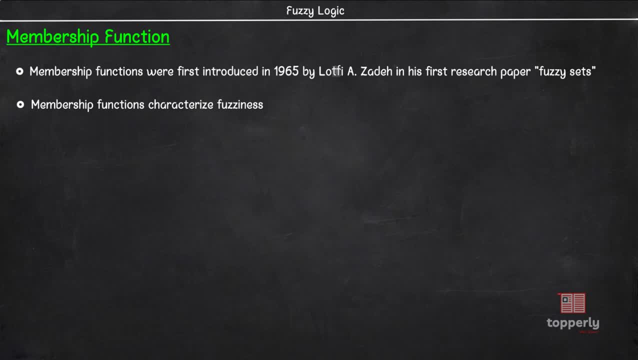 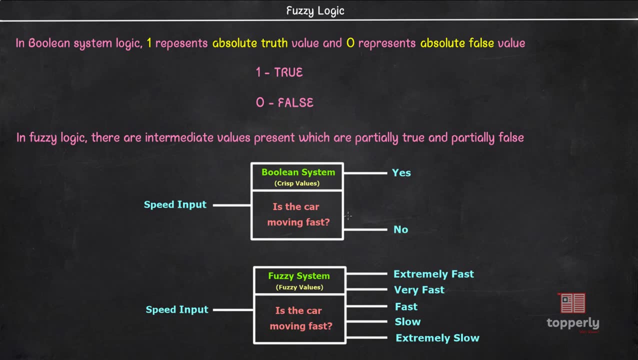 So essentially they represent the degree of truth in a system. For instance, in the previous example, for a Boolean system having CRISP values, the solution no represents absolute false value. Therefore the membership value over here is zero, Whereas in the case of true value, which is yes, the membership value is 1.. 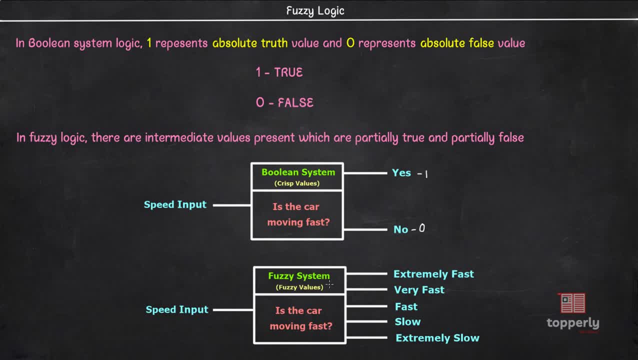 Coming to the case of Fuzzy Logic systems, it is somewhat different, Since we are dealing with partially true and partially false values. we may have membership values like 0.9, 0.8,, 0.6,, 0.3 and 0.1.. 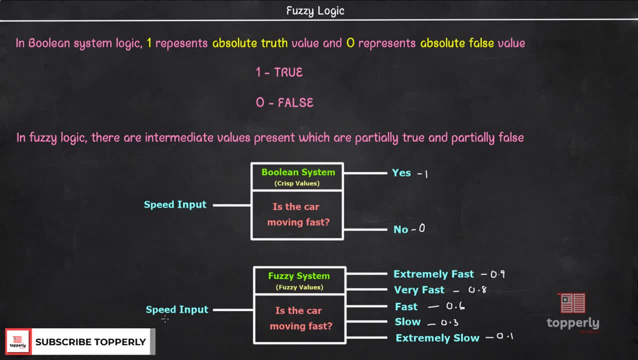 Now these values are assigned based on the degree of truth in the Fuzzy input with respect to the Fuzzy sets. As you can see that extremely fast is more close to absolute true value, So I have assigned it a value of 0.9, which is close to 1.. In similar fashion, extremely 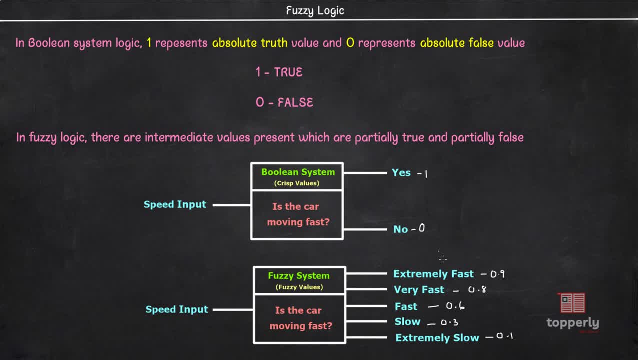 slow is close to the absolute false value. Therefore, I have assigned it a value of 0.1, which is close to 0.. So this is how Fuzzy Logic systems take up partial values and for each partial output they will be having a membership value assigned to it. 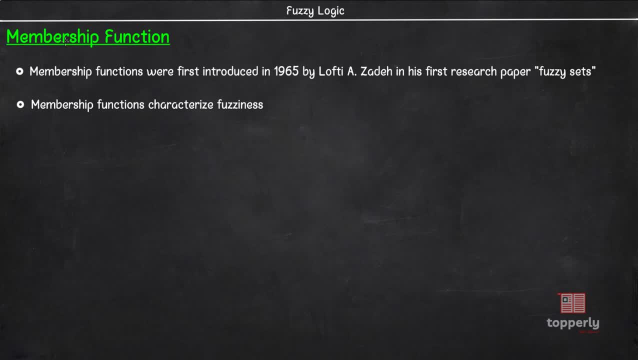 Therefore you can say that Fuzzy Logic systems are governed by membership functions. Let us now move on to Introduction to Classical Sets. A classical set is a collection of distinct objects and it has CRISP values, For example, a set of marks of students with marks above 75. So if you write this as a, which is a classical set? 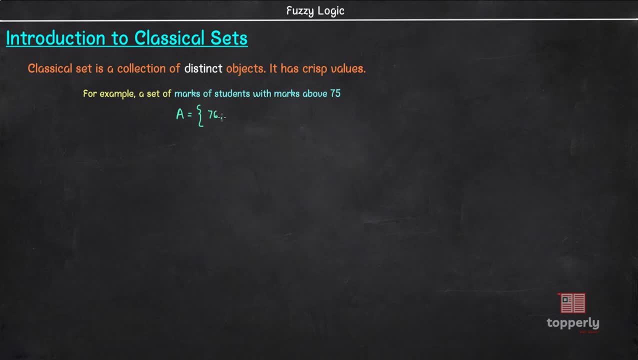 then a can have values such as 76,, 80,, 90,, 95 and so on. Now each individual entity in a set is called a member or an element of the set. That is, 76,, 80,, 90,, 95,. 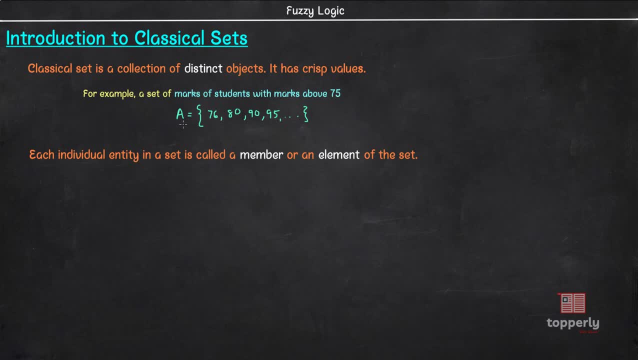 are called as elements or members of the set A. Therefore you can say that the classical set is defined in such a way that it has two groups: members and non-members. Here all the marks above 75 comes under the members of set A, But any mark which is less than or equal to 75,. 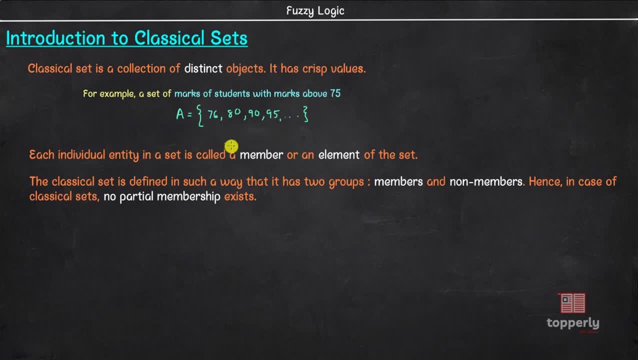 they are called the non-members of the set A. So you can say that in the case of classical sets, partial membership does not exist. There are only members and non-members. Now let S be a classical set. The membership function that can be used to define the set S is given by chi S of X. 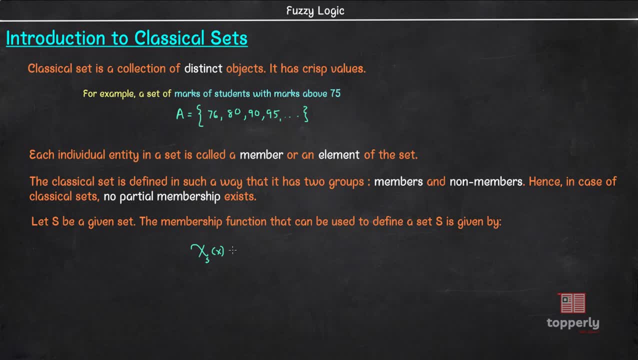 where chi is used to denote a classical set is equal to 1 when X belongs to S and 0 when X does not belong to S. So this is the definition of the classical set S In our example, set A. an element belongs to set A if its value is greater than 75 and the membership value for 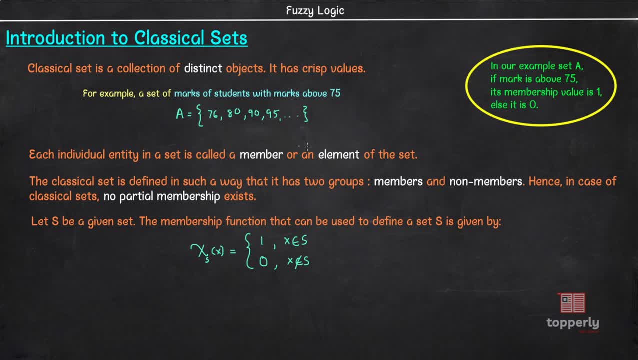 all elements belonging to set A is 1.. That is, chi A of 76 is equal to 1, chi A of 80 is equal to 1, chi A of 90 is equal to 1, and so on. In similar fashion, if we take chi A of 40, we know that the 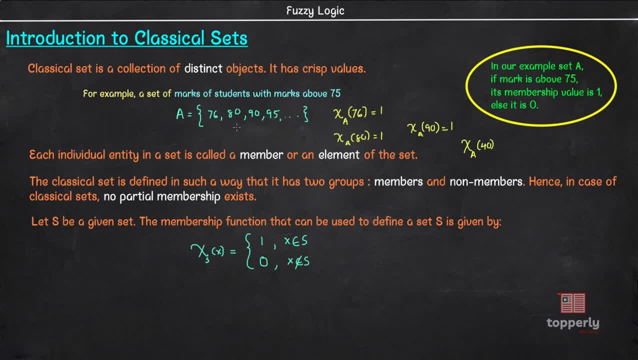 value 40 is not an element of set A, So chi A of 40 is equal to 0, because the membership value for non-members is 0.. Now, another important concept that you need to learn is cardinality. Cardinality of a set is the number of members belonging to a set that is greater than or equal to 0. So 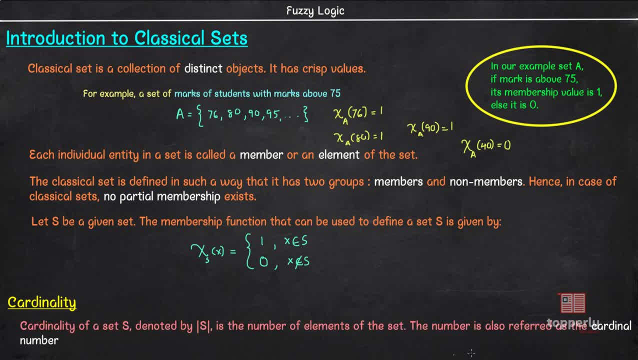 cardinality of a set is the number of elements of the set, and this number is also referred to as cardinal number. Let us take an example. Suppose you have a set B and it has elements A, B, C and D, Then you can say that the cardinality of set B is 4.. Why? Because there are 4 elements. 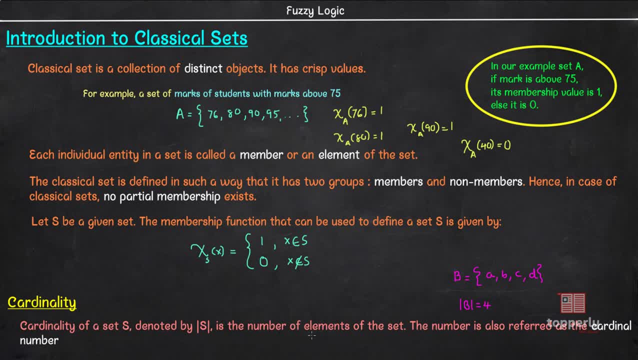 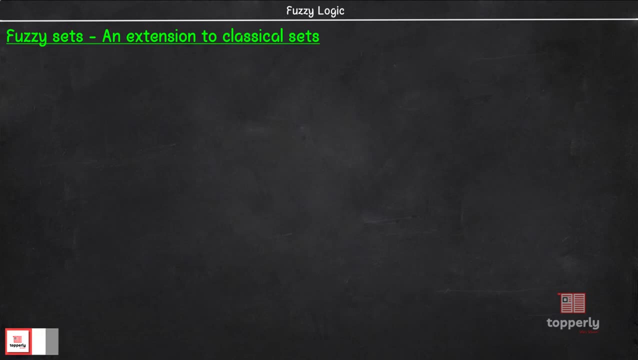 in the set. Therefore, in short, the total number of elements of a set constitutes cardinality, and in this example the number of elements is 4.. Therefore, the cardinal number over here is 4.. Now we will move on to fussy sets and extension of classical sets. 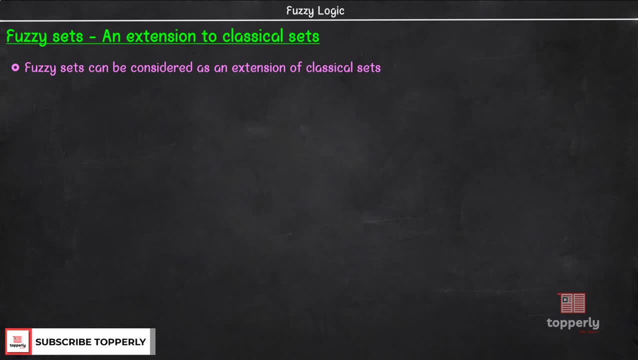 Fussy sets can be considered as an extension and a gross oversimplification of the classical sets. We can understand fussy sets in the context of set memberships. Basically, it allows partial membership, which means that it contains elements of a set that is greater than or equal to 0.. 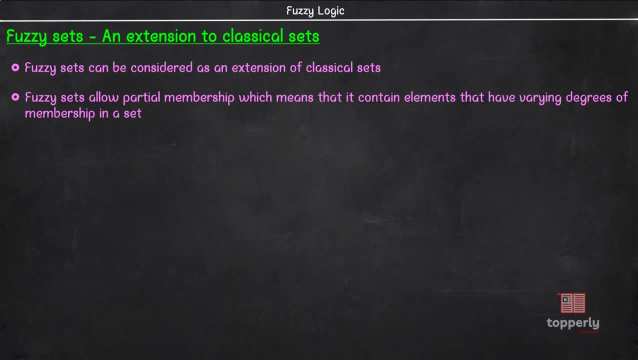 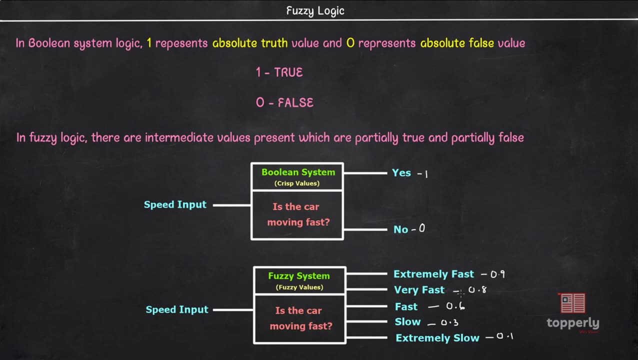 Fussy sets are set of elements that have varying degrees of membership in a set. Now in the previous example under fussy logic systems we have seen varying degree of membership like 0.9, 0.8,, 0.6, 0.3 and 0.1 in various fussy sets. So 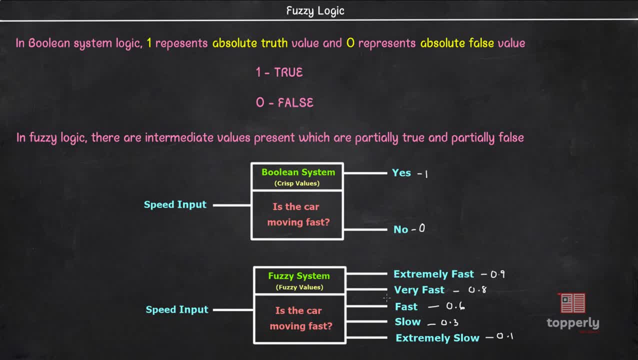 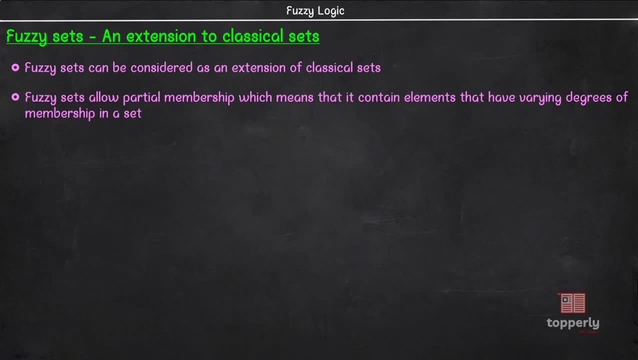 these represent the partial values and they constitute the degree of membership of the input element in each of these fussy sets particular line. Now we can understand the difference between classical sets and fussy sets. Classical set contain elements that satisfy precise properties of membership, while fussy 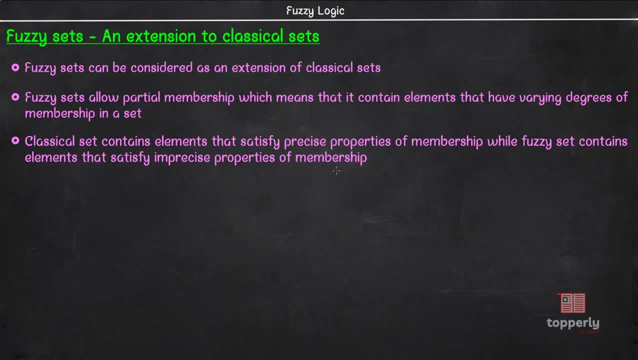 set contain elements that satisfy imprecise properties of membership. This property becomes more evident when you see the graphs for fussy set and classical set. So let us consider two graphs, one for fussy set and one for classical set. As you have learned just now, the membership value. 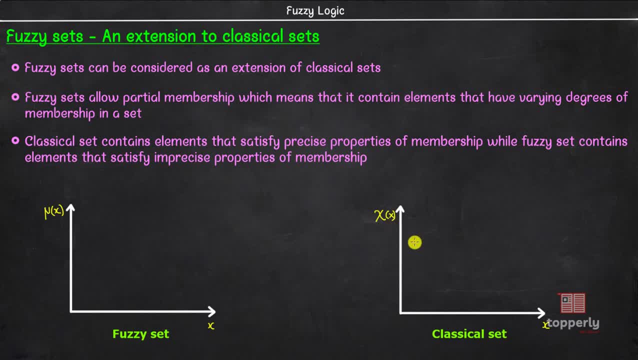 for a classical set is denoted by chi of x and x. over here is the element. In similar fashion, the membership value for a fussy set is denoted by mu of x. We will learn about it in a bit. Now, the graph of a fussy set may look like this, whereas the graph of a classical set. 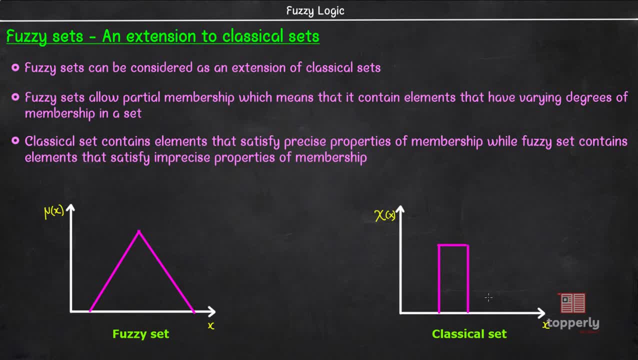 is denoted by mu of x. Now, the graph of a fussy set may look like this, whereas the graph of a fussy set may look like this: The graph of a fussy set looks like this because these particular regions over here. they represents the partial membership values. Partial membership values. 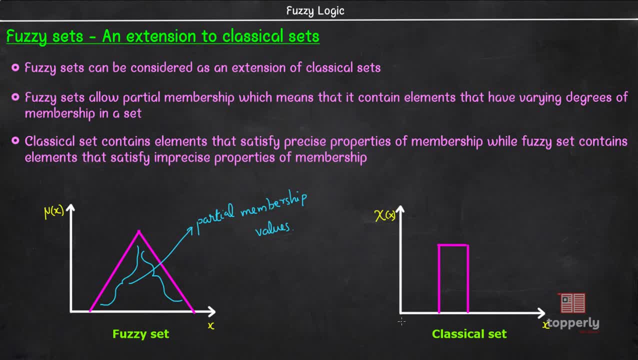 But in the case of classical set, we are only allowed to have 0 and 1.. Therefore, you get a graph like this. You will understand this better when we discuss examples later in this video Coming to the mathematical definition of fussy sets. a fussy set a. 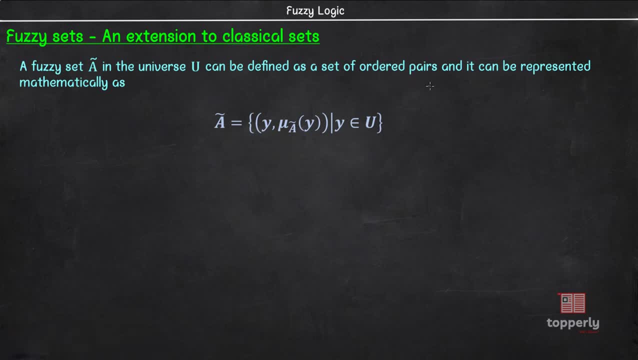 in the universe. U can be defined as a set of ordered pairs and it can be represented mathematically as a, where this tilde sign denotes that a is a fussy set, is equal to ordered pair y, mu A of y, where y is the element or value and mu? a of y is the membership function and u is. 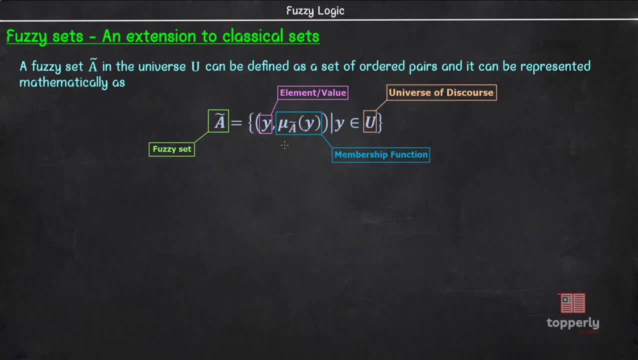 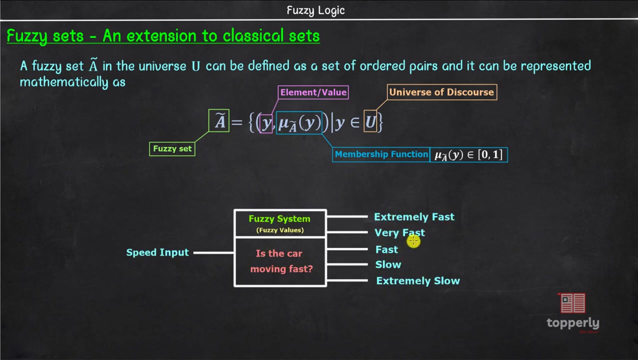 the universe of discourse. An important point to note here is that the value of mu a of y lies in the range of 0 to 1, with 0 and 1 included In our example discussed earlier. extremely fast, very fast, fast, slow and extremely slow. these 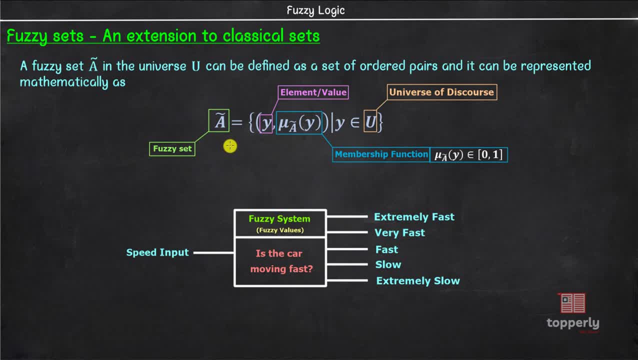 are the different fussy sets, just like our set A, and we can represent these sets on a fussy graph as a function on a speed scale. So let us do that, Okay. so I have an x-axis which represents speed and a y-axis which represents 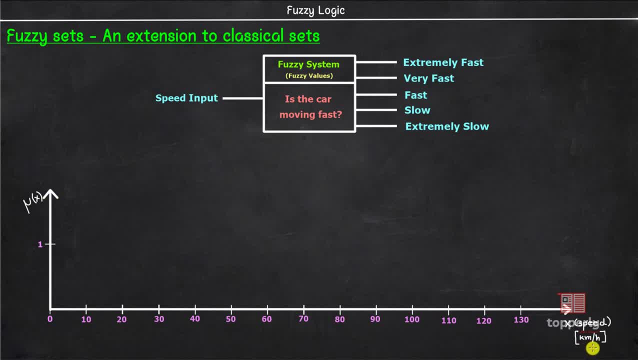 membership value. As you can see, x-axis has speeds marked in kilometer per hour. Now let us try to map our fussy sets into this graph. Now, everyone agrees that any speed below 10 kilometer per hour is an extremely slow speed. 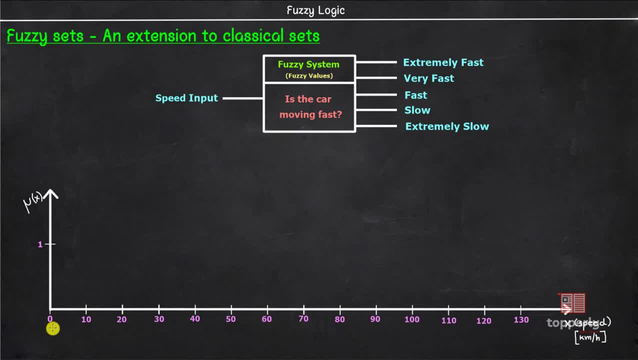 right, That means all the speeds between 0 and 10 kilometer per hour are members of the set extremely slow. Okay, since everyone are in agreement that these speeds are extremely slow, we can give the membership values of these speeds here: us 1 in the set, extremely slow, So we can write that mu extremely slow of 0 km per hour is equal. 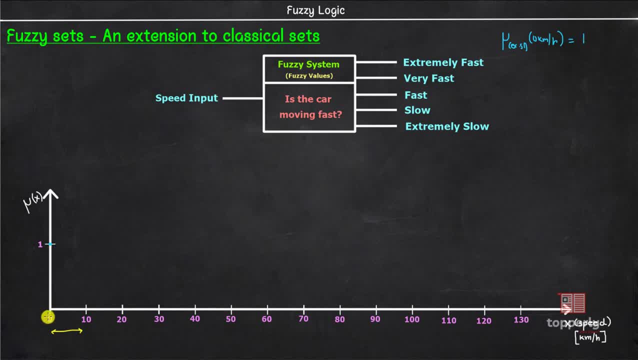 to 1. that is, the membership value of 0 km per hour is 1 in the set. extremely slow, Now, similarly mu extremely slow- of 1 km per hour is also 1.. So the membership value of 1 km per hour is 1 in the. 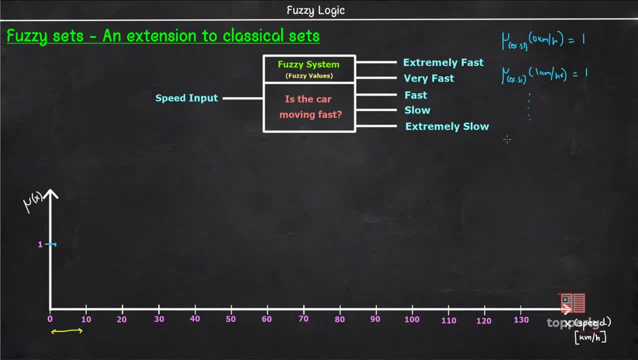 set extremely slow, Likewise all the speeds up to mu extremely slow. 10 km per hour is 1.. Therefore, the membership curve for the fussy set extremely slow has membership value equal to 1 for all the speeds in the range of 0 to 10 km per hour. Okay, now the question is: what about 11 km per hour? Does that belong to the? 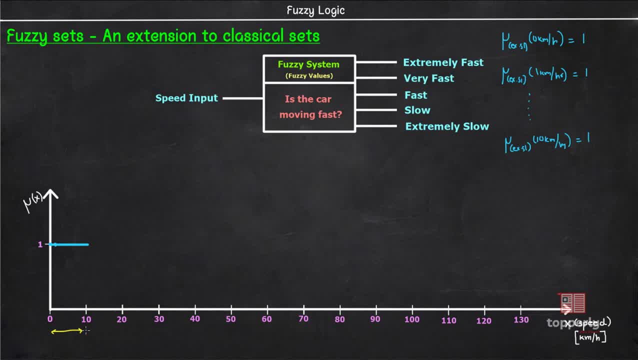 set extremely slow. Well, 11 km per hour is definitely faster than 10 km per hour, but it is still pretty slow, right? So we say 11 km per hour is not a full member of the fussy set extremely slow, but it is a partial member and let's say, 90 percent belongs to it, So we can write. 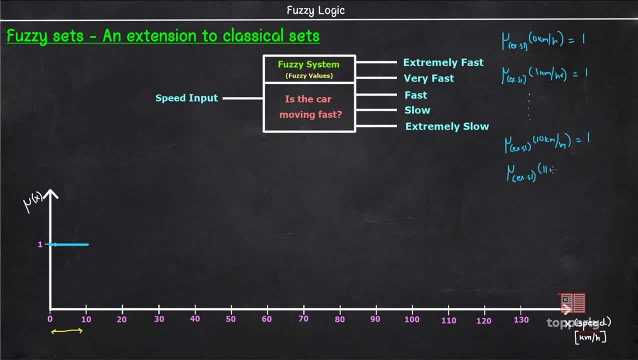 mu extremely slow- of 11 km per hour is equal to 0.9. that is the speed. 11 km per hour has a membership value of 0.9 in the fussy set extremely slow. Let us mark it on the graph. So 0.9 lies somewhere here. 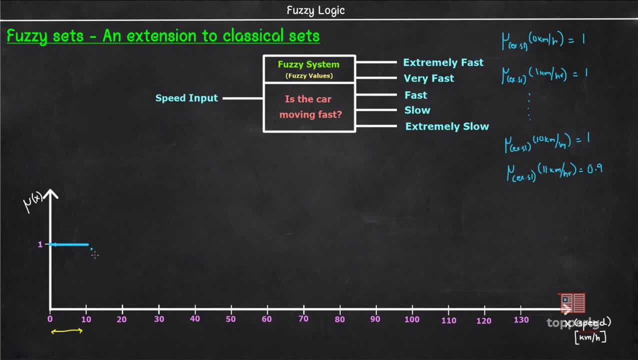 Now, using similar arguments, we can say that 15 km per hour is only a 50% member of the set. extremely slow, So mu, extremely slow. 15 km per hour is equal to 0.5 and let us mark it on the graph. 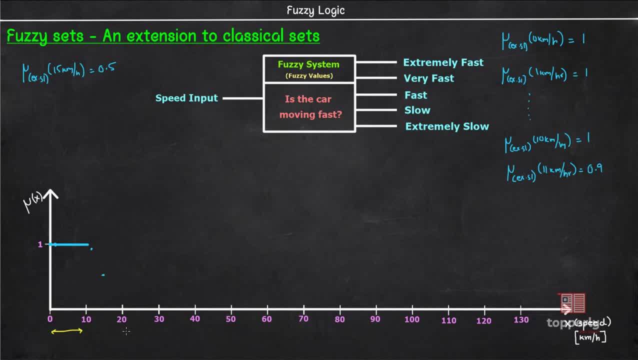 What about 20 km per hour? We can all agree that 20 km per hour is not an extremely slow speed anymore, So we can write mu extremely slow. 20 km per hour is equal to 0. That is 20 km per hour. 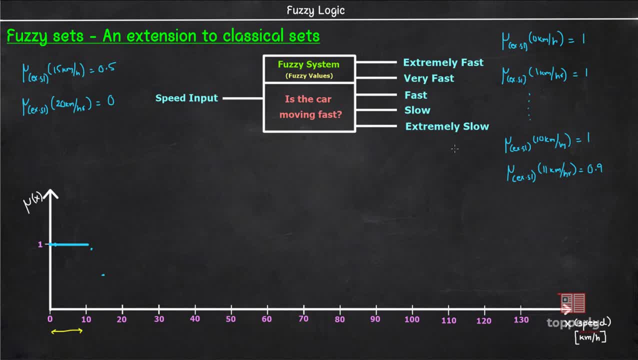 does not belong to the set extremely slow. Therefore, our fussy set extremely slow can be like this: And the membership value of all the speeds above 20 km per hour is also 0 in the fussy set extremely slow. Therefore, we get a flat line like this: Okay, so let us write this down This: 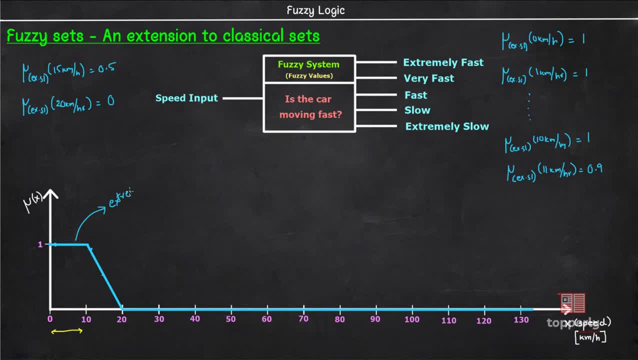 blue graph represents the fussy set extremely slow. Now, using the same arguments, I am mapping the fussy set slow. Let us say the same argument is used for the fussy set extremely slow. So we can say that the speeds in the range of 20 to 30 km per hour are full members and the speeds in 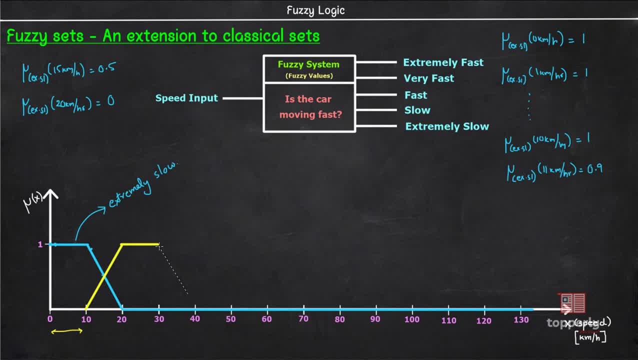 the range of 10 to 20 and 30 to 40 are partial members And the membership value is 0 for all other speeds. Okay, by the way, I chose this speed range randomly. You are free to choose your own range of speeds for the fussy set slow. So this represents the set slow. 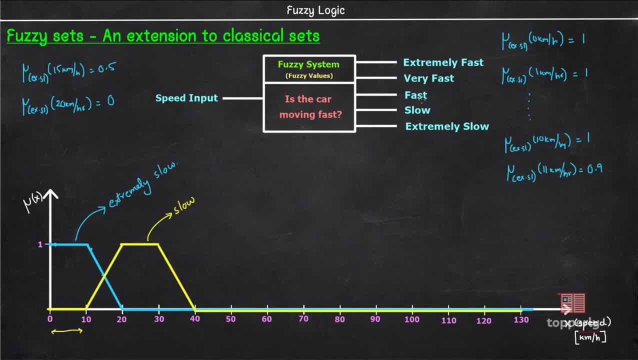 Now, in similar fashion, I will draw the fussy set fast. So we have our fussy set fast, So this is fast. Next, we have very fast, This is very fast. Finally, we have extremely fast, A lot of time has, So extremely fast. 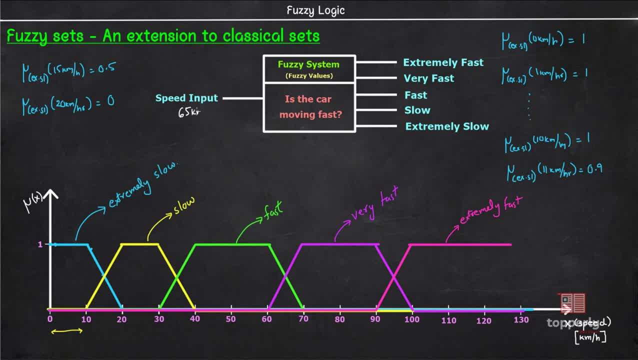 Now, if we give a speed, say 65 km per hour, as an input to our fuzzy system, it will give out the membership value of 65 km per hour in each of these sets. So, based on the curves we defined, the membership value of 65 km per hour is zero in the fuzzy. 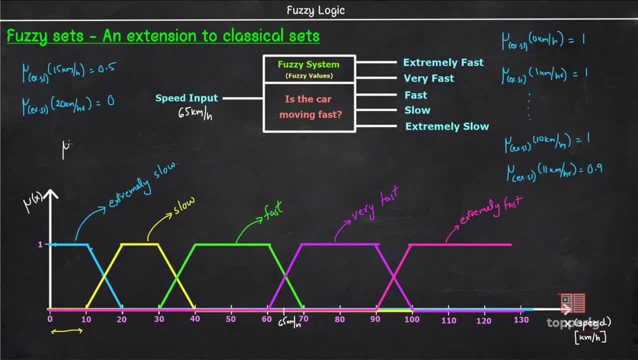 set extremely slow. So mu extremely slow of 65 km per hour is zero. We can write that down here also. Similarly, the membership value of 65 km per hour in the fuzzy set slow is also zero. So mu slow, 65 km per hour is also zero. 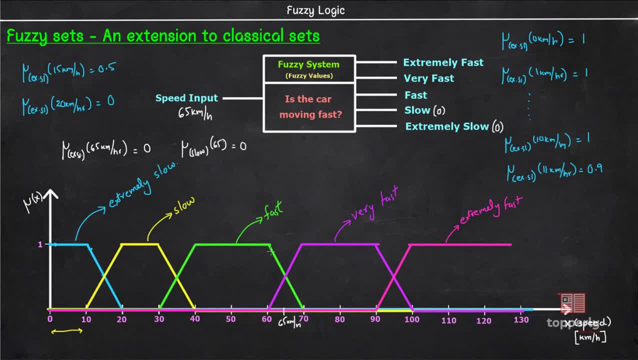 But when it comes to the fuzzy set fast, we can see that 65 km per hour is a partial member and its membership value is 0.5.. Therefore, mu fast 65 km per hour is 0.5.. Here also 0.5.. 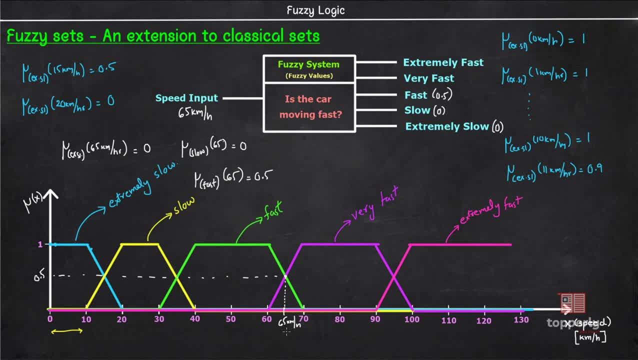 If you check again You can see that 65 km per hour is 0.5.. So mu very fast of 65 km per hour is also a partial member of the fuzzy set very fast. Here also, the membership value is 0.5.. 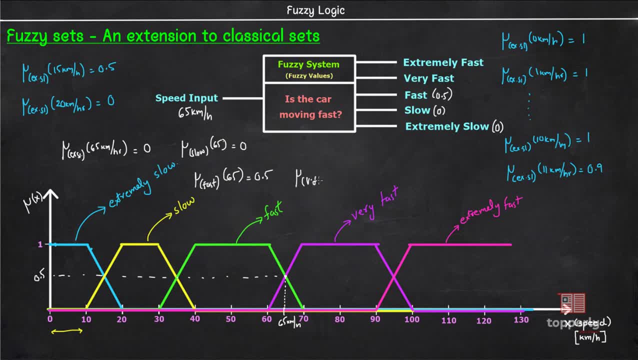 Therefore, mu very fast of 65 km per hour is 0.5.. We can write that down here also. Finally, as you can see, 65 km per hour is not a member of the fuzzy set extremely fast. Therefore, mu extremely fast, 65 km per hour is 0.5. 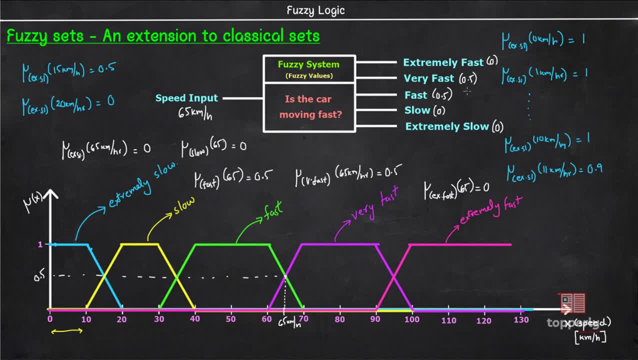 Here also, we can write it as 0.5.. Okay, so I hope you got a general idea of what a fuzzy set is and what are membership values. One important point to remember is that there are many curves used to define fuzzy sets. Here we have used trapezoid shaped curves. 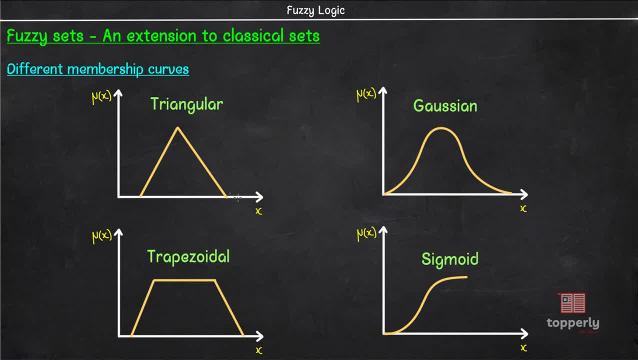 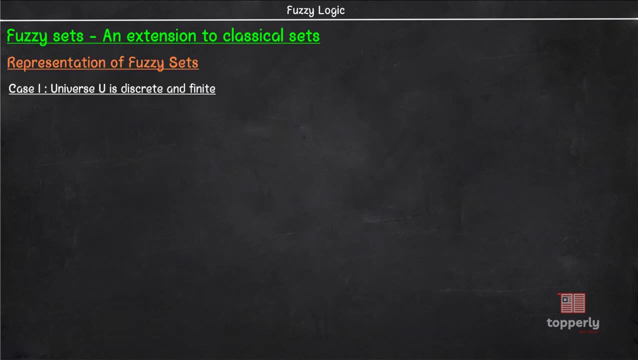 Earlier, we have seen triangular shaped curves. We can also define fuzzy sets using sigmoid or Gaussian functions. Therefore, we should choose the type of curve which suits our application. Okay, Now coming to the representation of fuzzy sets. There are two ways to represent them. 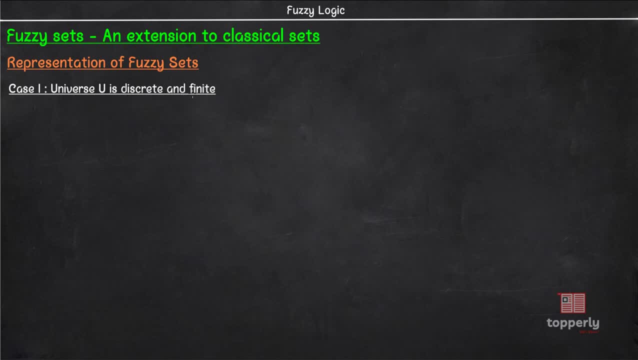 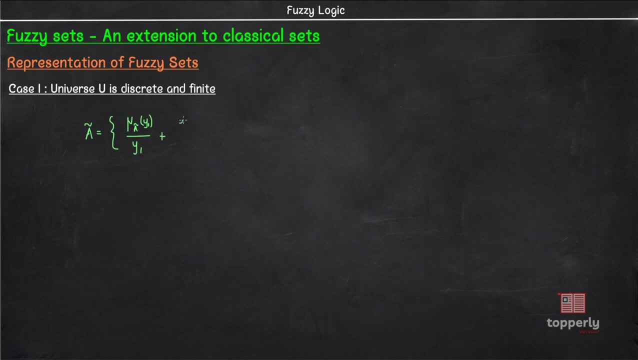 Membership value of y1 in fuzzy, set A by y1.. Membership value of y1 in fuzzy, set A by y1.. Membership value of y2 in fuzzy, set A by y2.. Membership value of y3 in loadin. in order to understand the background, 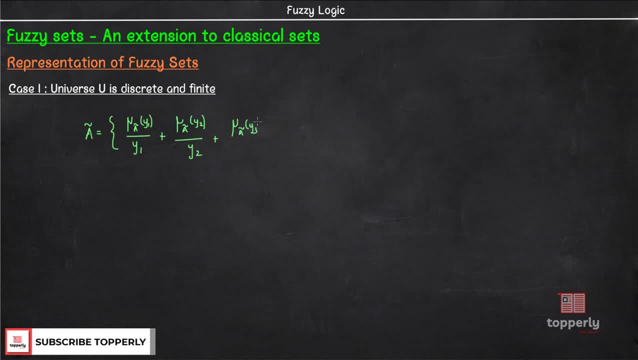 Plus Moscow to Utah is Versus 12, With a number less than or equal to 1 plus membership value of y2 in fuzzy set A by y2.. Versus 12 plus the list of slightly smaller memberships as above, Verses y1, site y2, site y3, and site y1 are elements of a fuzzy set A. 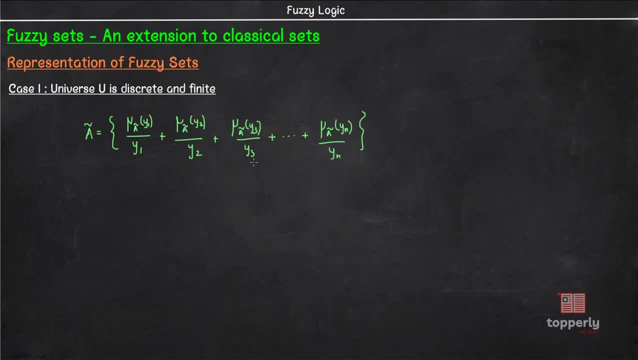 Verses y1, land and seat y2, site y3, and site y3 are elements of a fuzzy set. A ítulo represented as sigma i, equal to 1 to n membership value of yi by yi. An important point to note here is that these plus signs does not mean actual 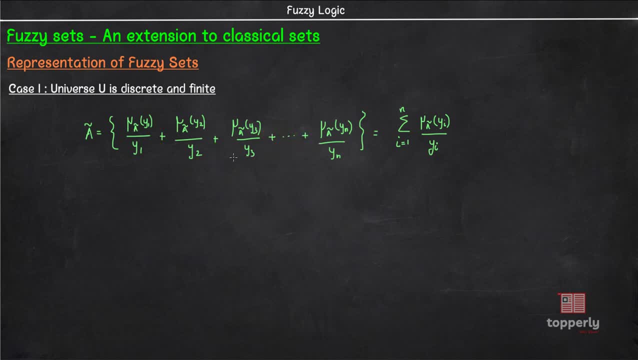 addition, They are just a representation symbol for the collection of elements of y. Same is the case for these symbols: They are not actual divisions or fractions. Okay, There is one more way to represent the same fuzzy set A. It can be written as A equal to ordered pair of y1: membership value of y1 in A comma. 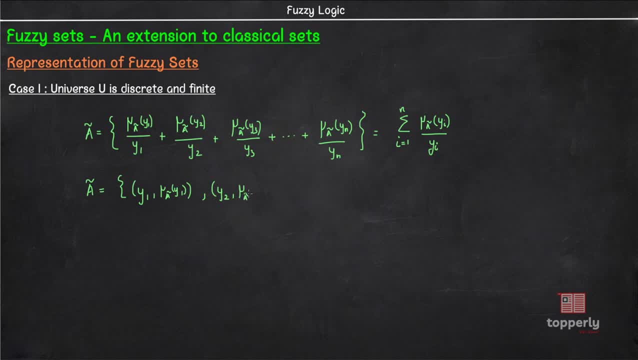 ordered pair y2. membership value of y2 in A, etc. till yn comma. membership value of y2 in A comma. membership value of y2 in A comma. membership value of y2 in A comma. membership value of yn in A. Okay, So these are the two ways to represent a. 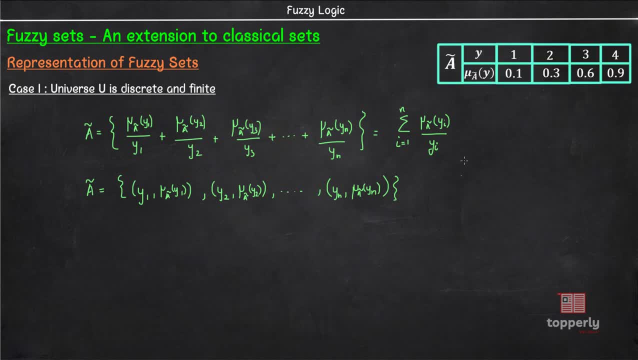 fuzzy set. Let us take an example so that this concept is clear. Suppose we have a fuzzy set A with four members- 1, 2, 3 and 4- and the corresponding membership values of members is 0.1, 0.3, 0.6 and 0.9.. Using the first representation, we 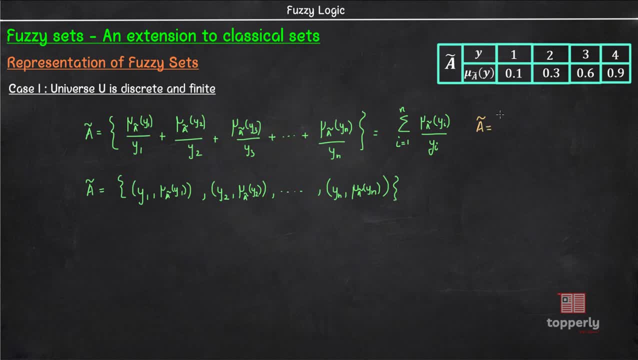 learned fuzzy set A can be written as membership value of element 1, which is 0.1 by element 1, plus membership value of element 2, which is 0.3 by 2 plus 0.6 by 3 plus 0.9 by 4.. Now, using our second way, 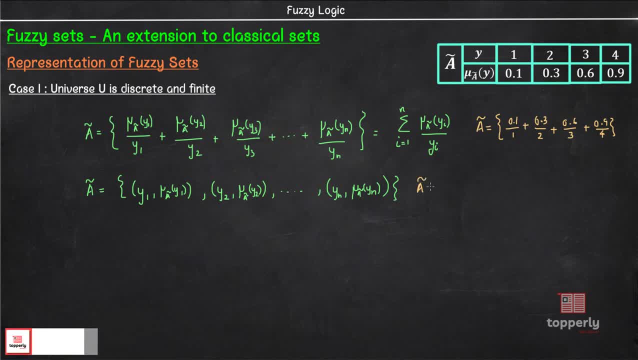 to represent the same fuzzy set A can be written as 1.1, 2.3, 3.6 and 4.9, that is, as ordered pair of element and its membership value. Next, when it comes to universe U, which is continuous and infinite, we will: 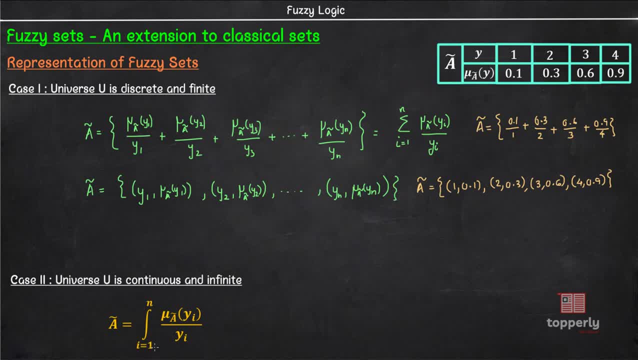 replace the summation symbol with the integral symbol, that is the sum of the member functions inside the interval set A. The integral symbol and its members are not inextricably linked, so the sum of them are still an integral. So theN null I, theN pro of ever is equal tommorh aMuA 3, fl2 i vs mu's- Pedigree in case, if we divide by the number of object participants, theR Meth of the Become 이번uister Member calls manifest it. This set represents the collection of each element in the set. Now, before ending the lecture, let us see a small example to show how crisp and Fuzzy set representations differ for the same situation. Let's remember you will useимости and needs to create some of the random choice whenever we want to create very complex situations. Remember, always being balanced is more efficient than false in these situations. Let's, Sir, go through with our Subscribe tool. 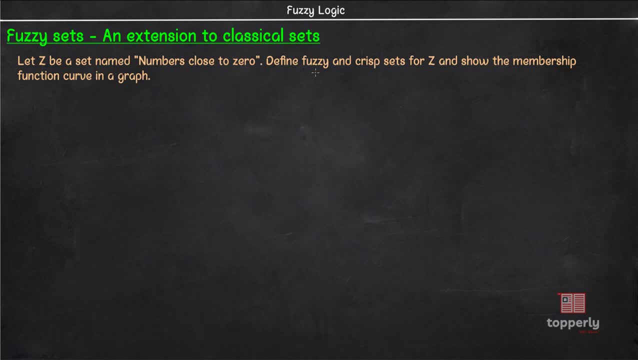 be a set named numbers close to zero, Define fussy and crisp sets for set and show the membership curve in a graph. Okay so let us first define a fussy set. We will use a triangular curve for this- which is centered at zero, like this This: 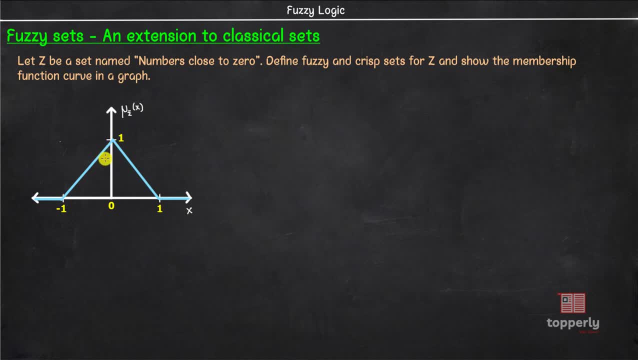 curve makes sense right, As you can see, numbers close to zero has high membership values and the membership value progressively decreases on either side as we move away from zero. Now that we have finalized the membership curve, let us define the curve mathematically So we can write: mu: set of x equal to: 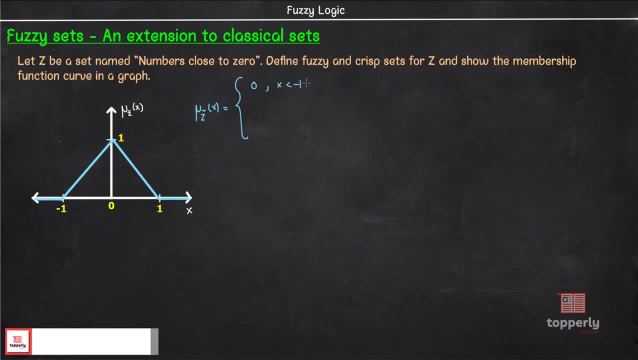 zero. when x less than minus 1, which is clear in this graph Coming to this region, the equation of the straight line is y equal to x plus 1.. Since here y axis is mu of x, we can write the same function as the function of negative x. So we can define: 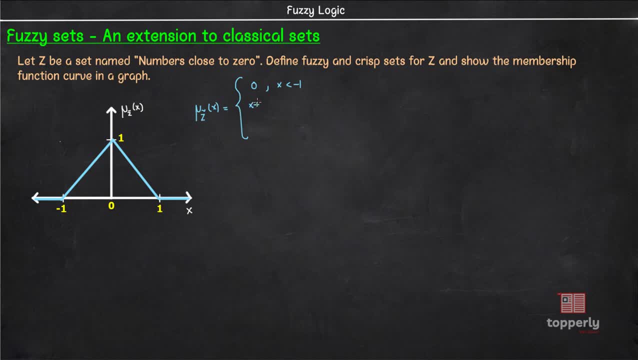 can write mu of x equal to x plus 1. for minus 1 less than or equal to x less than 0.. Similarly, for the region between 0 and 1, we have x minus 1, 0 less than or equal to x less than 1 and is equal. 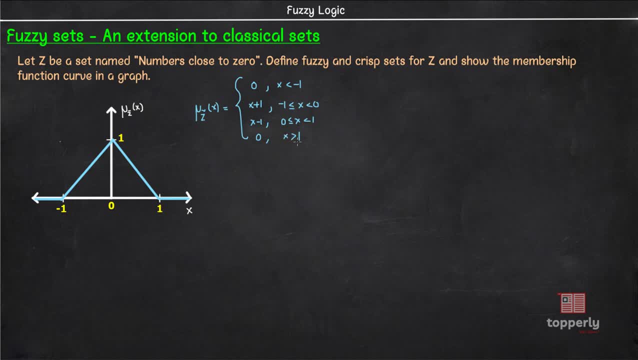 to 0 when x is greater than 1.. So this is the membership function for the fuzzy set set which we have defined here. Alternatively, we can also use Gaussian function to define another fuzzy set for z like this: This curve can be mathematically written as: mu z of x equal to e, raised to minus. 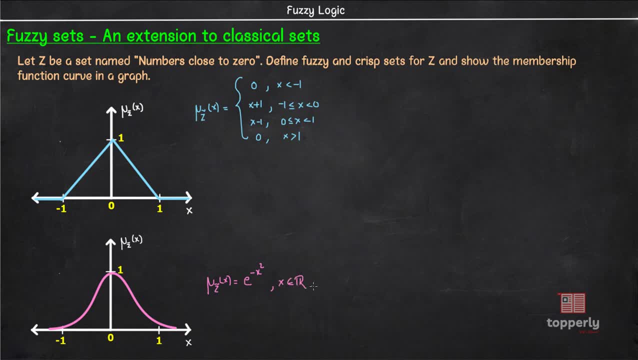 x square where x belongs to r. So this is another membership function for the set z. Here you should note that even though both these members are the same, membership functions are used to characterize the same description: numbers close to 0.. Both of these are different fuzzy sets, So ideally we should use different labels, like mu, z1 of x. 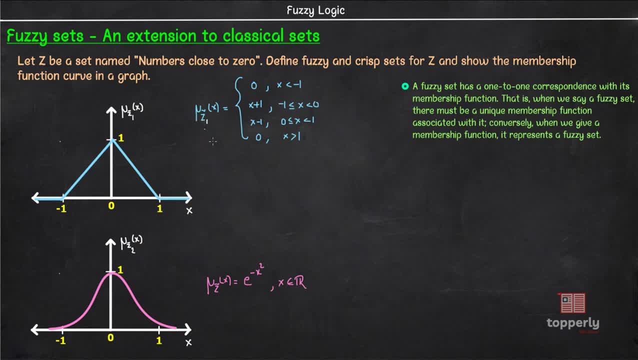 and mu, z2 of x here, Here also z1 and z2.. Okay, another important point to note is that the properties that a fuzzy set is used to characterize are usually fuzzy. For example, numbers. Numbers close to 0 is not a precise description right. Therefore we may use different membership. 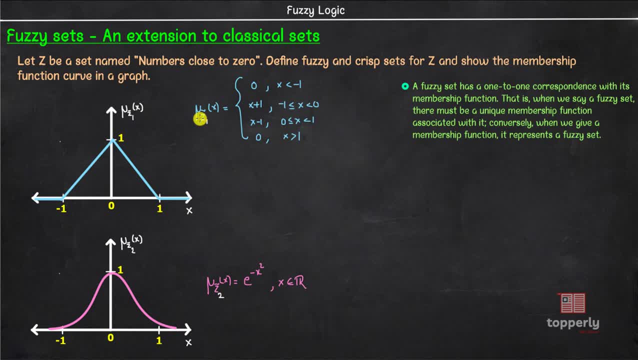 functions to characterize the same description. But the membership functions defined are not fuzzy themselves. They are precise mathematical functions. So you can see that once a fuzzy property is represented by a membership function, nothing is fuzzy anymore. Therefore, by characterizing the fuzzy description with a membership function, we have to know the 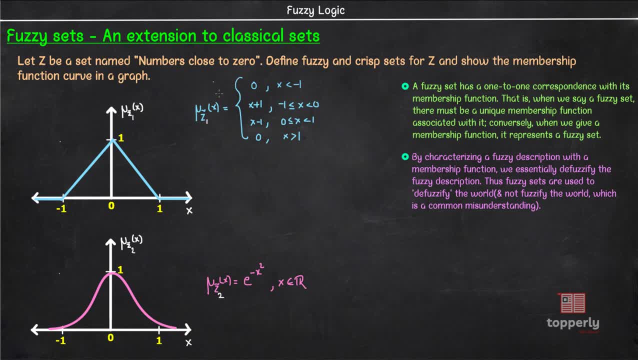 function of the membership function. All the safety measures are at the same place. we have actually defuzzified the fuzzy description. A common misconception many of us have is that Fuzzy Set Theory tries to Fuzzify the world. But what I explained just now shows otherwise. 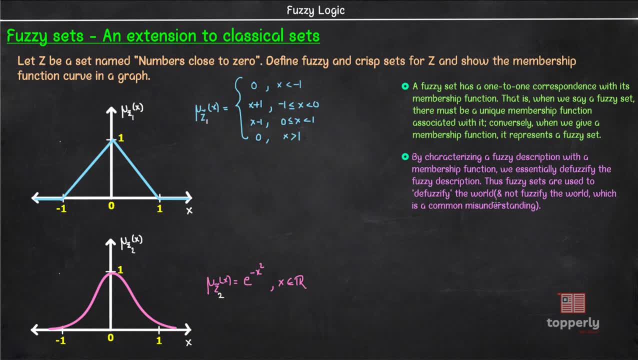 Fuzzy Sets are used to De-Fuzzify the world. Ok, now a doubt many of us will be having is how to determine the membership function curves. Well, sadly, there is no one way to do it. one approach is to talk with experts, but sometimes it is difficult because there are so many. 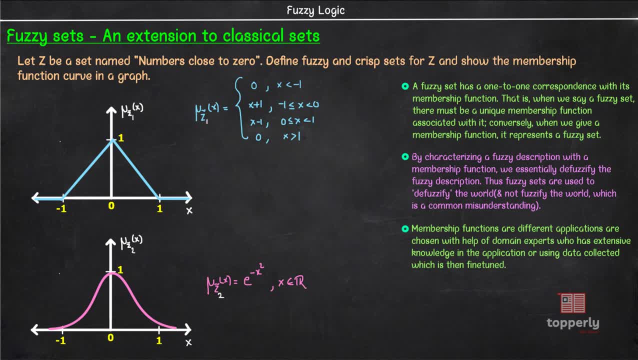 methods to solve them, But never we are left sandwiched between two concepts: This new approach to talk with experts in the field and use their knowledge to create a membership function. Another approach is to gather lots of data related to our application and use that data.